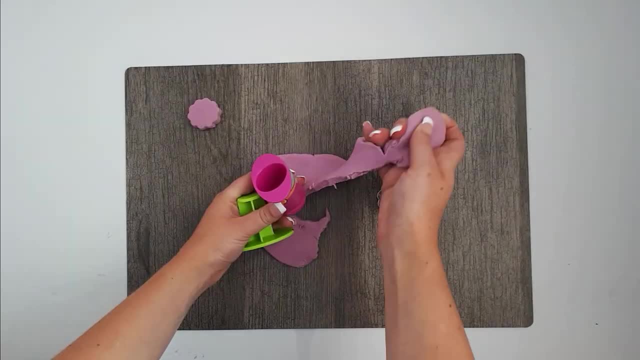 cream of tartar, And then I added the cream of tartar And then I added the cream of tartar of dry and that the salt granules were falling out. I guess it just goes to show you that just because something is very popular on the internet doesn't necessarily mean it's. 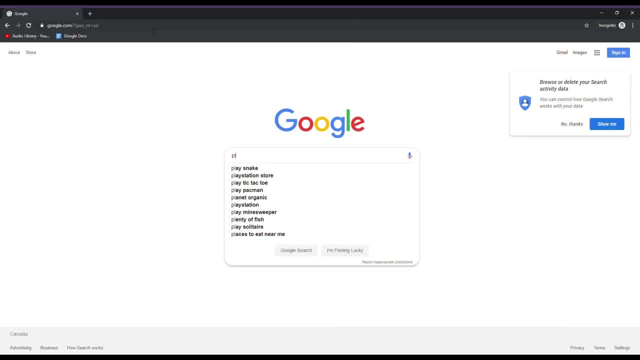 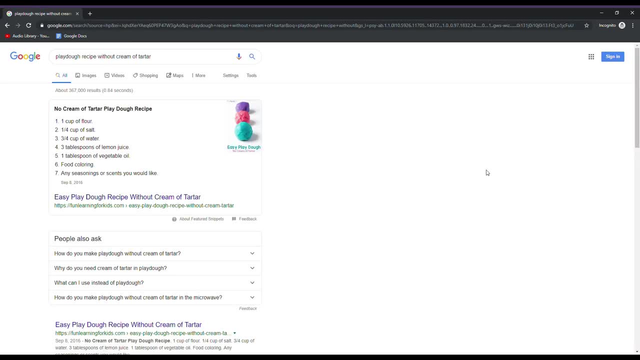 the best. I'm glad we tried it, but I wouldn't remake it again. Next up was a recipe that holds the number one spot on Google, and that is the easy Play-Doh recipe without cream of tartar by funlearningforkidscom. This recipe will need to be cooked on the 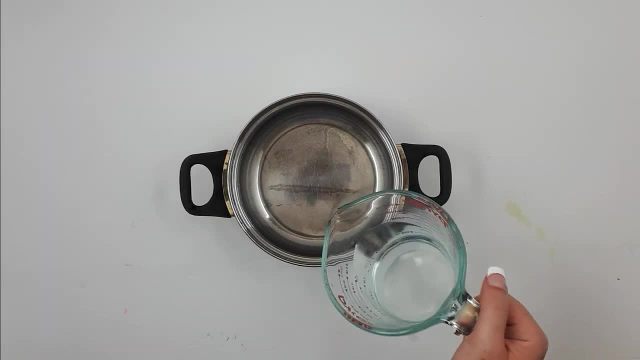 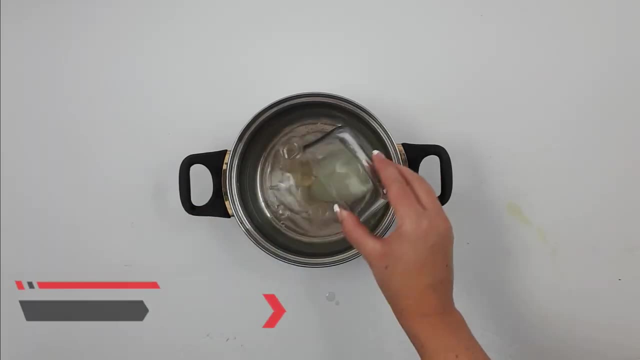 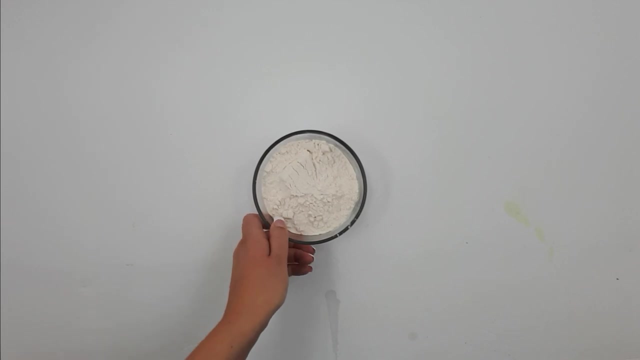 stove, so I added my wet ingredients directly into a pot. The recipe called for 3 quarts of water, 1 tablespoon of vegetable oil, 3 tablespoons of lemon juice and I added 10 drops of food coloring. In a separate bowl, I added 1 cup of flour and 1 quarter cup of. 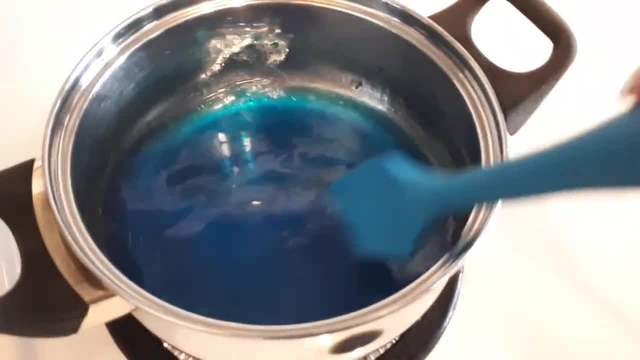 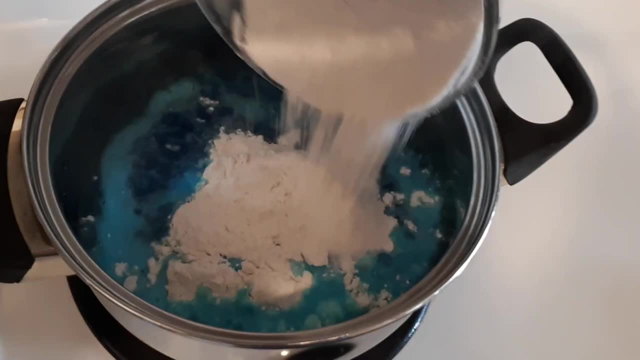 salt and I mixed it together. Next, I put my pot on the stove and heated it on medium. When it was hot but not boiling, I added the dry ingredients. You can see here. I just dumped the entire bowl in. It was just really hard holding the camera at the same time, but in 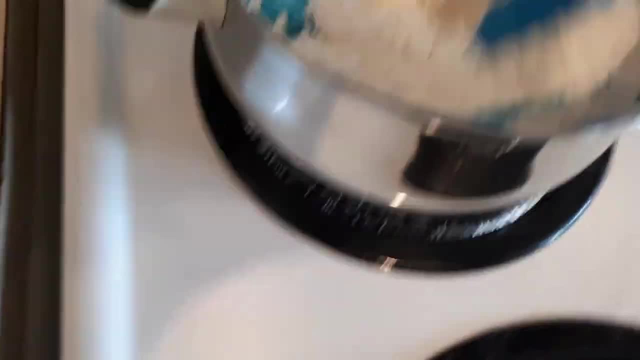 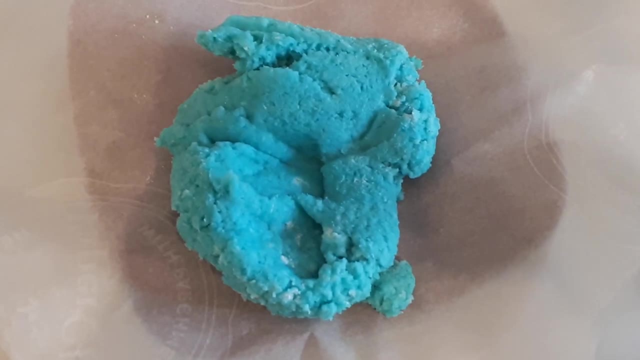 the instructions she does say you don't need to heat it up. I stirred the mixture together until the Play-Doh was cooked and then dumped it out on a parchment-lined plate to cool. You can see it was a little lumpy at first because 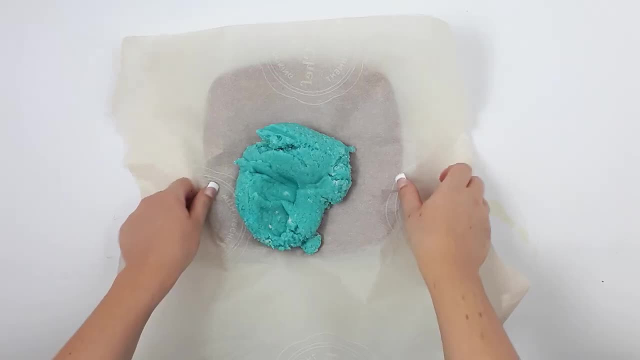 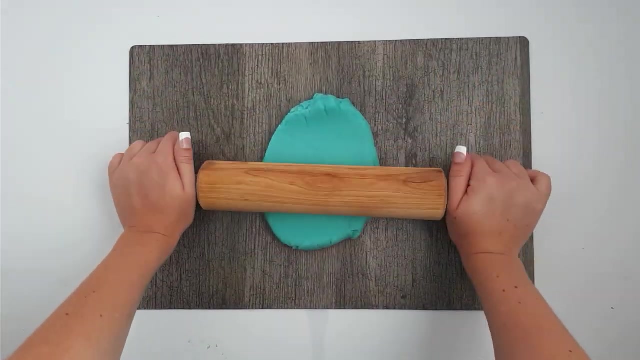 of how I added the dry ingredients, but you will see that it all smoothed out in the end. When the Play-Doh had cooled off, I began kneading it for a few minutes until it was nice and smooth. This recipe was the perfect mix between soft and squishy, but dense enough. 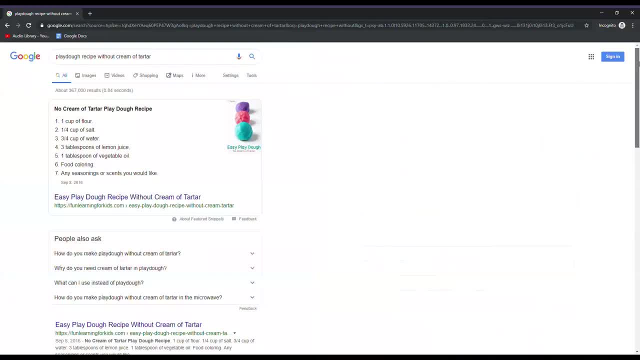 to hold its shape. It's something I will definitely make again Next up. I tried a recipe that ranks number two on Google, and that is the easy Play-Doh recipe without cream of tartar by funlearningforkidscom. This recipe was the perfect mix between soft 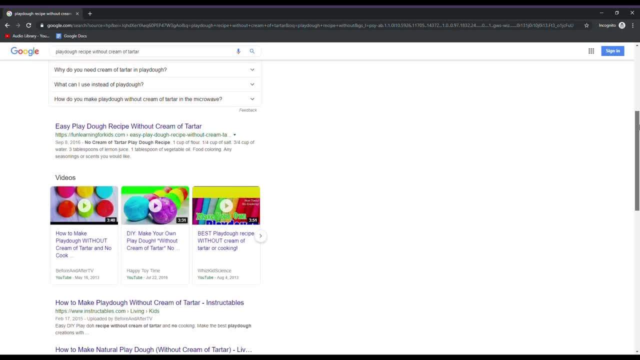 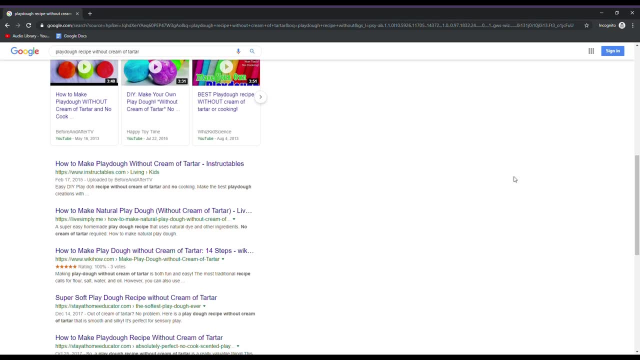 and squishy, but dense enough to hold its shape. It's technically in the third spot, but number two actually belongs to the first recipe we tried, so I'm calling it number two. This recipe comes from livesimplyme and is called natural Play-Doh without cream. 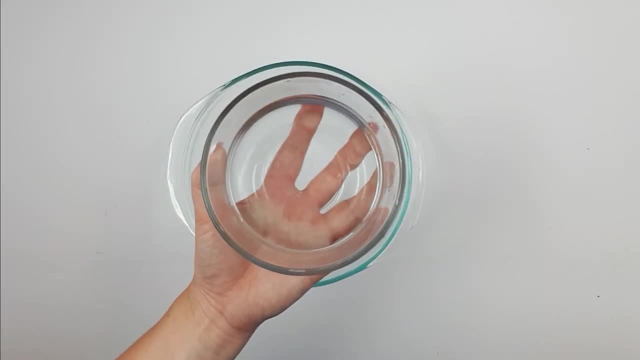 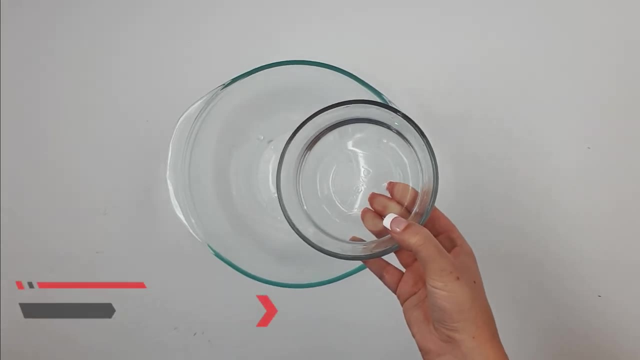 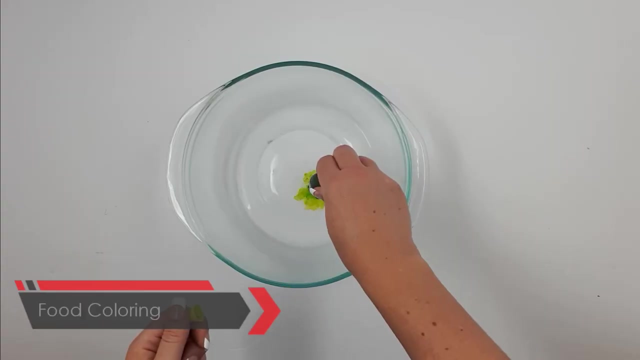 of tartar. This recipe is no cook, so no need for a pot this time. I just use a glass bowl. I adjusted her original recipe to make only one ball of Play-Doh, so my measurements were one half and one eighth cup of hot water, one tablespoon of olive oil and food colouring. 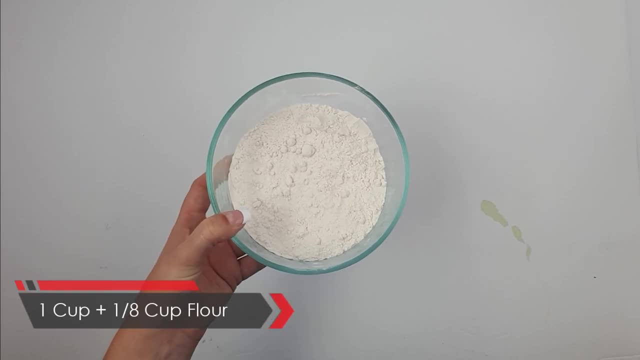 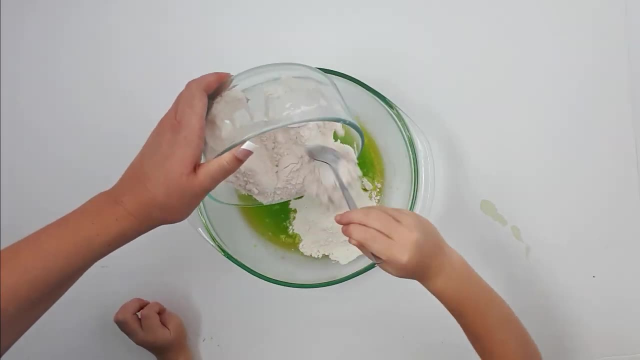 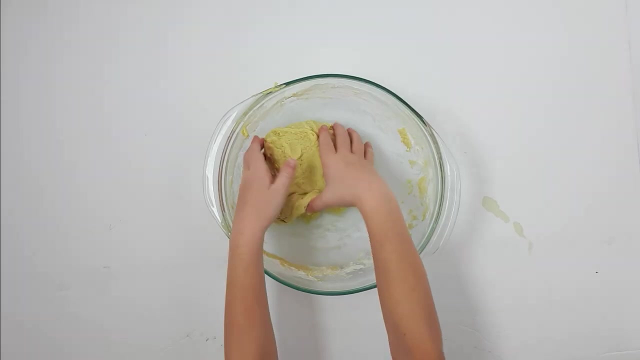 In a separate bowl, I added the dry ingredients, which were one and one eighth cup of white all-purpose flour and one half cup of salt. I added the dry ingredients to the wet and then gave it a stir. After stirring, I switched to using my hands and began to knead the dough. 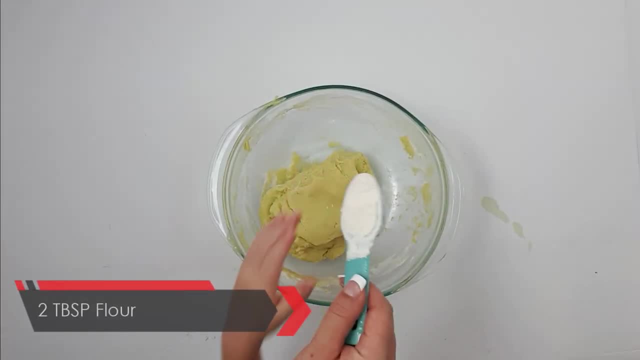 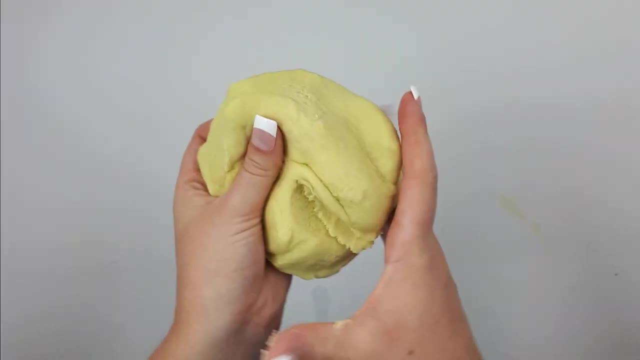 In the recipe she notes that she usually ends up adding an extra two tablespoons of flour. My dough was pretty sticky, so I went ahead and added those extra two tablespoons. Although this dough was super soft, it was still sticky after adding the flour and the 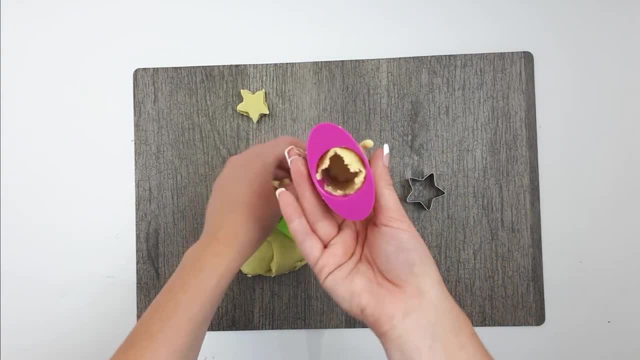 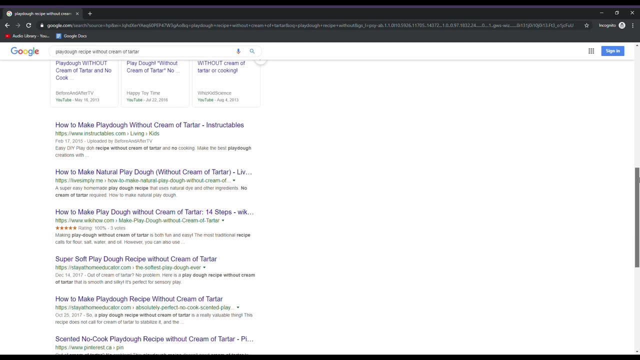 extra flour. I think, if I had played with the ratios a bit more, that it might turn out nice. but it was time to move on to our next recipe. The fourth and final recipe I tried is from stayathomeeducatorcom. This recipe does not. 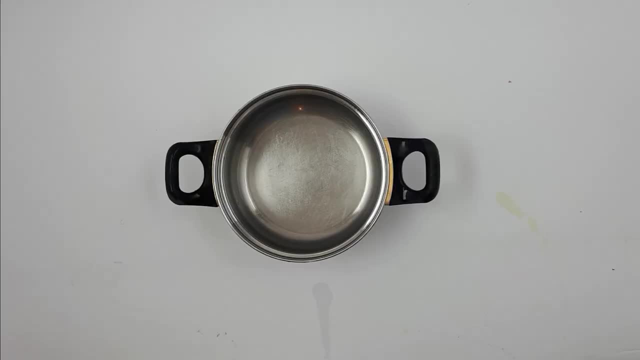 contain cream of tartar or salt, which I thought was unique. This recipe needs to be cooked, so I started out with my wet ingredients in a pot. I adjusted her recipe for one ball of Play-Doh. The measurements were one cup of water, one tablespoon of lemon juice, one. 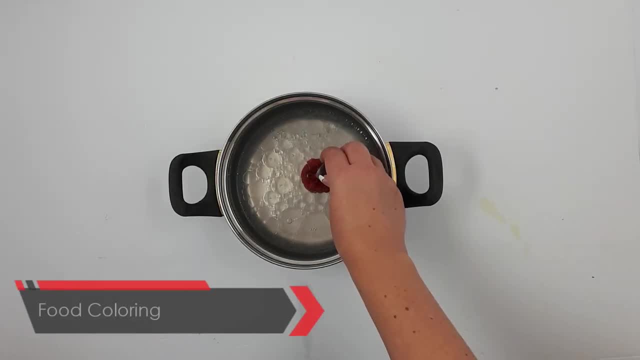 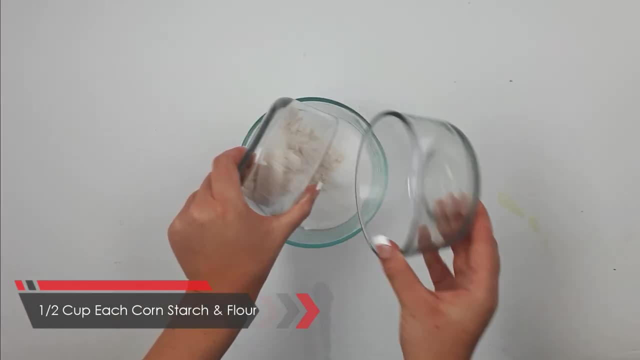 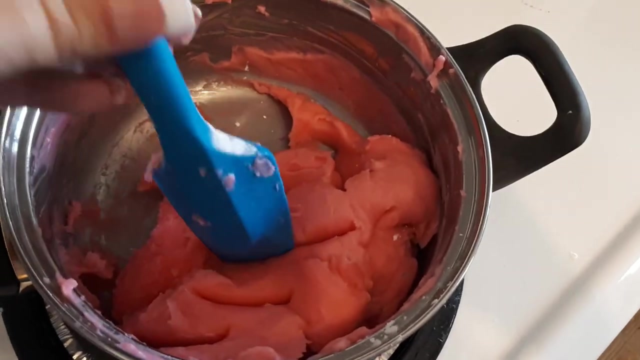 tablespoon of vegetable oil and food coloring. In a separate bowl I mixed my dry ingredients. They were one half cup of flour and one half cup of corn starch. Next it said to cook all the ingredients over low heat until the Play-Doh comes together. After that I dumped. 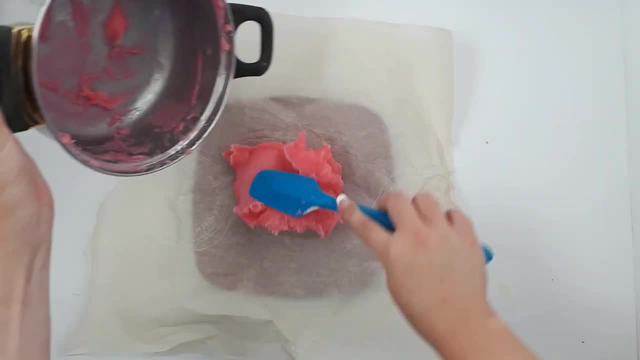 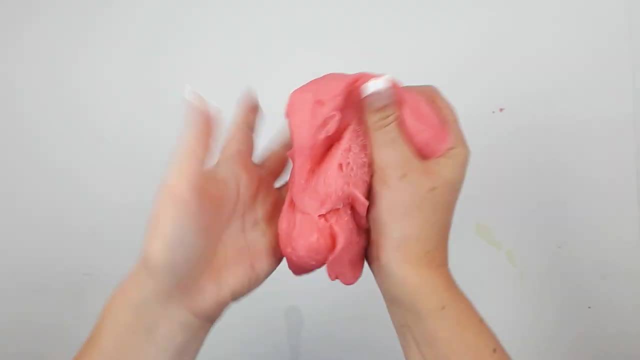 the ball into a parchment lined plate to let it cool When it was safe to touch. I kneaded it for several minutes until I had a smooth, squishy Play-Doh ball. On her post she writes that this is the darkest Play-Doh you will ever touch and thus far I would have to agree. 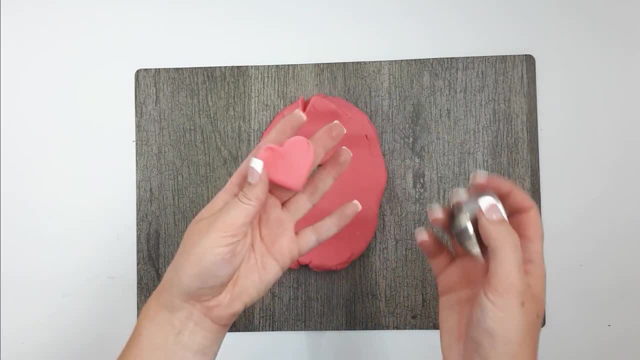 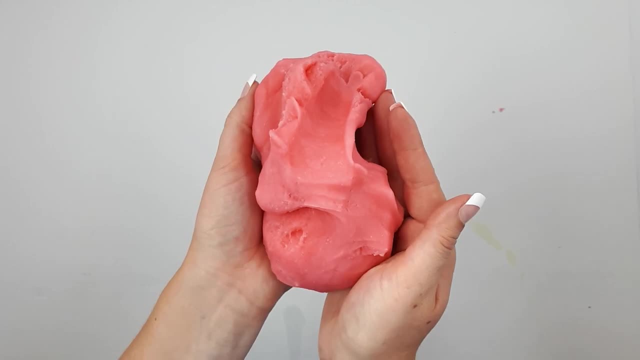 This Play-Doh is so fun and squishy to touch and I love that it doesn't require any cream of tartar or salt. Now for my final thoughts. Which Play-Doh recipe without cream of tartar is the absolute best? It came down to two contenders for me, and that was the blue Play-Doh I made from. 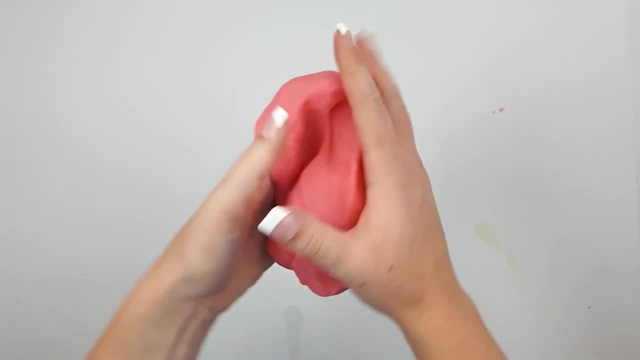 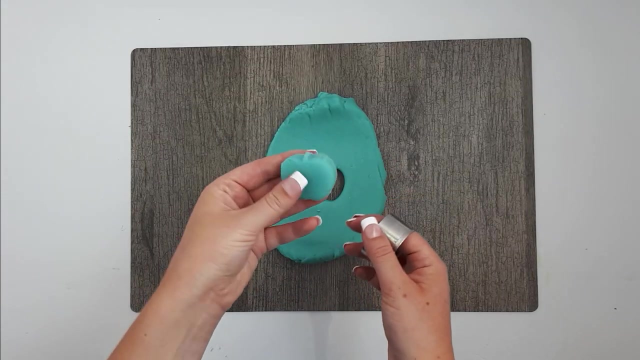 Fun Learning for Kids and the pink Play-Doh from Stay at Home Educator. After playing with both for several weeks, I noticed some minor differences. The blue Play-Doh is slightly more dense, so it holds its shape a little better than the pink Play-Doh.